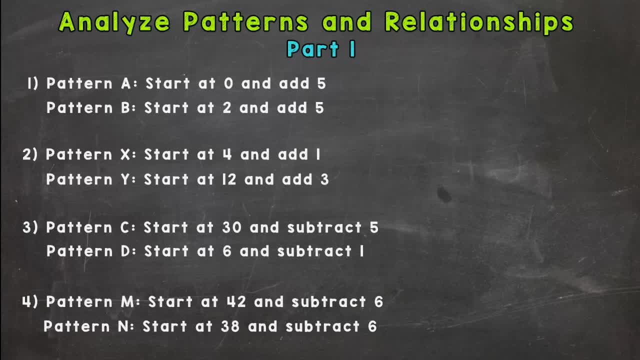 I highly suggest writing these out with me as I go through. I think that will be beneficial to you learning this. but if you just want to watch and listen, that's okay too. So we're going to hop into Number 1 here and see what's going on with these patterns. So we have 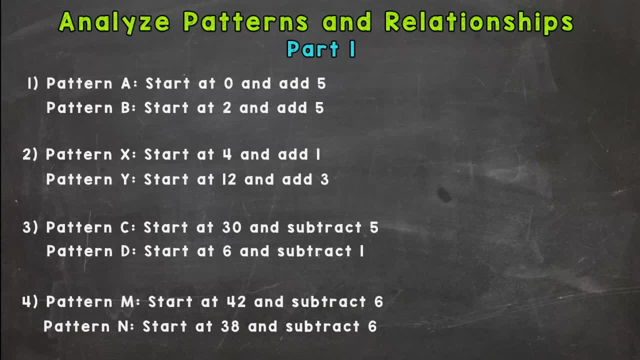 Patterns and Relationships, Part 1.. So we're going to hop into Number 1 here and see what's going on with these patterns. So we have Pattern A and Pattern B. We're going to do one at a time and we need to be nice and neat when we line these up. That is key. So let's start with Pattern A and 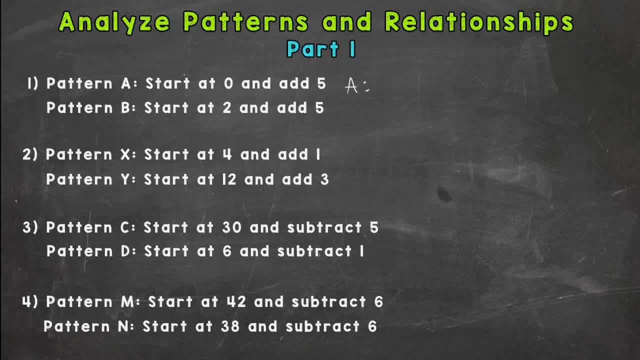 I'm going to write in A, so I have my pattern labeled here And all I need to do is follow directions. It says: start at 0 and add 5.. So guess what? you start with 0.. Imagine that And add 5 each time: 0,, 5,, 10,, 15,, 20.. 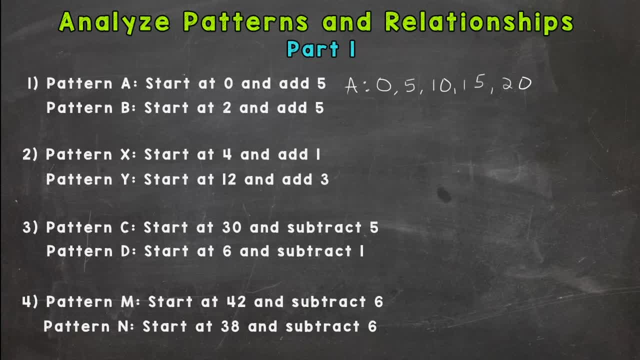 That pattern goes on forever, but no need to continue on. We'll end it at 5 terms Terms is a very important vocab word. Terms are just the numbers you write out in your pattern. So 0 is the first term, 5 is the second, 10 is the third, 15 is fourth And I bet you you got the hang of 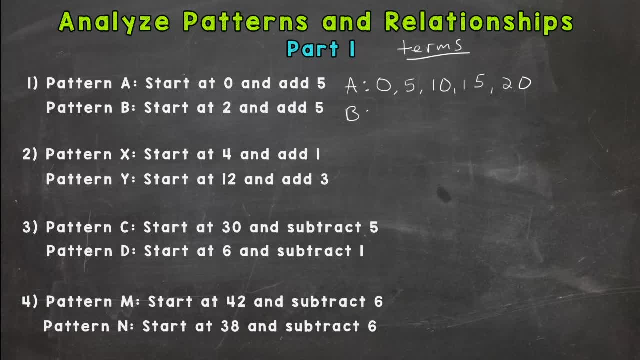 it. So let's do B here. So Pattern B: we start at 2,, not 0.. Don't start at 0.. Don't start at 0.. Don't start at every pattern with 0.. You have to pay attention to what you're doing and follow the direction. So 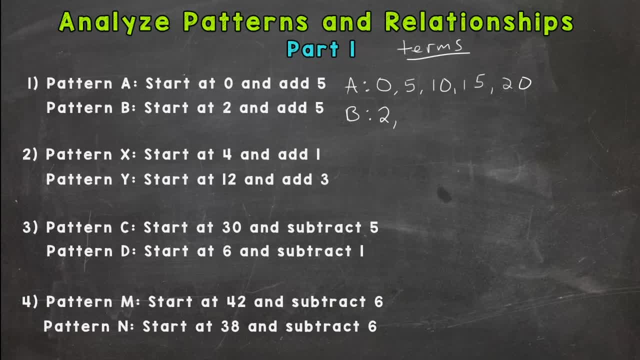 it says: start at 2.. Add 5 each time, So 2,, 7,, 12,, 17, and 22.. Those are our terms for Pattern B. Now notice the patterns A and B are lined up. The first terms are lined up right above and below. 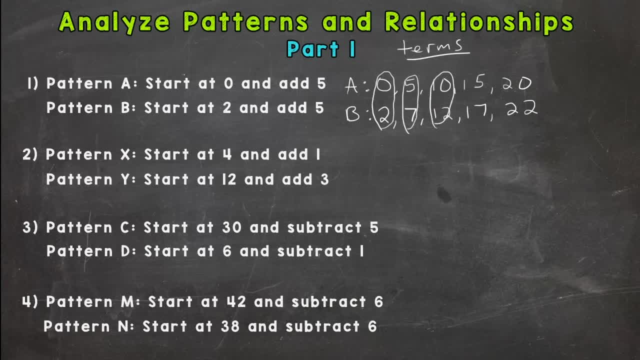 each other. So we're going to start at 2, not 0.. Don't start at 0.. Don't start at 0.. Don't start at 0.. The second terms are lined up: 3rd, 4th and 5th. So now that we have our patterns written, 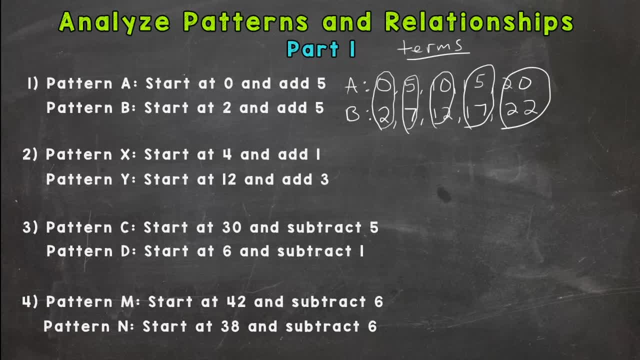 out. we need to see the relationship between A and B. How do we get A to equal B? And it needs to work for all of them like a rule. So we have a 0 and a 2. Think, add, subtract, multiply. 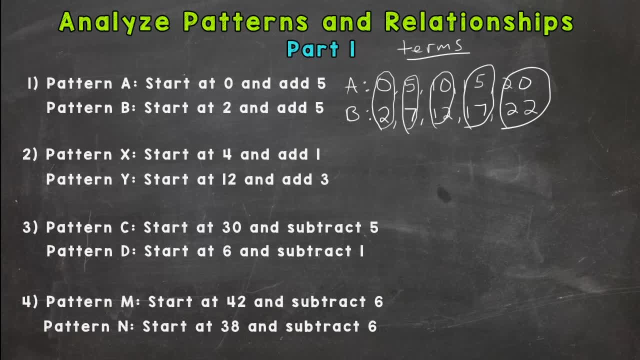 or divide. Those are your four options. So how do we get 0 to equal 2?? You're probably thinking to yourself: well, add 2 to 0.. Okay, so let's try it. 0 plus 2 is 2.. It works for. 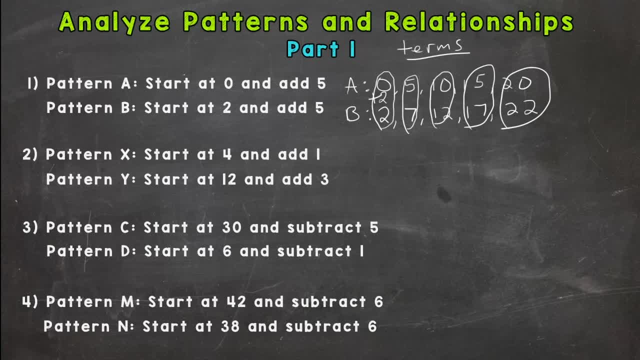 the first term It needs to work for all of them, Never just check 1.. At least check the 5 you have and if you write even longer patterns, check all of them. Make sure it works for all. 5 plus 2 is 7. Works. 10 plus 2 is 12.. 15 plus 2 is 17.. 20 plus 2 is 22.. It works. 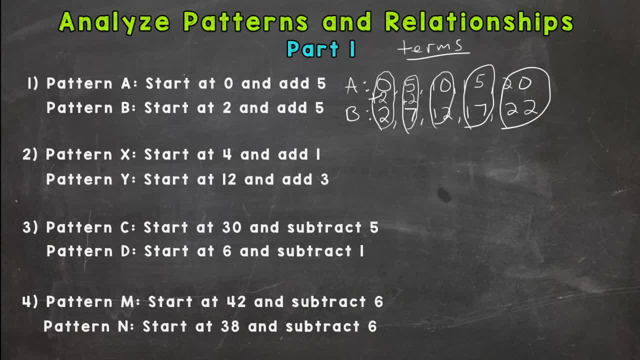 for all 5 of those. so pretty safe to say here that the rule or relationship is: adding 2 to pattern A will give us the corresponding terms in pattern B. Now this is a new vocab concept here: Corresponding terms, And that means the first terms in the patterns A and. 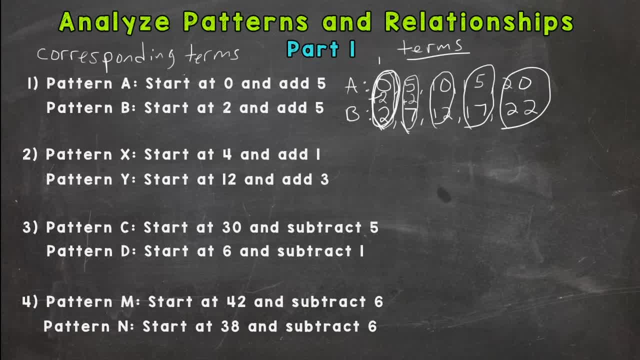 B. these guys are like partners, They're corresponding terms And that means the first terms in the patterns A and B are corresponding terms, The 5 and 7, the 10 and 12, and so on. So those are corresponding terms. So you'll see a lot of different types of answers to these. You 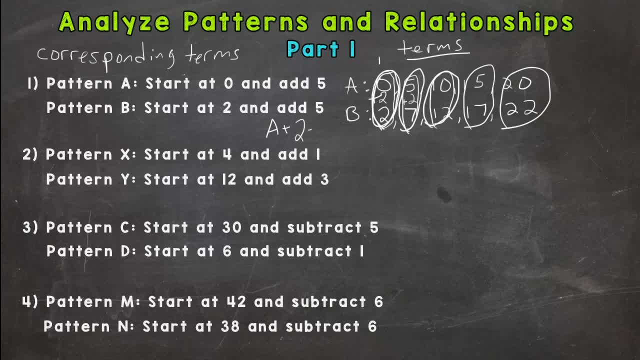 can write it out as a math problem like: A plus 2 will give you pattern B, something like this, Or maybe you'll have to do it in sentence form and it will go something like: pattern A plus 2 will equal the corresponding terms. 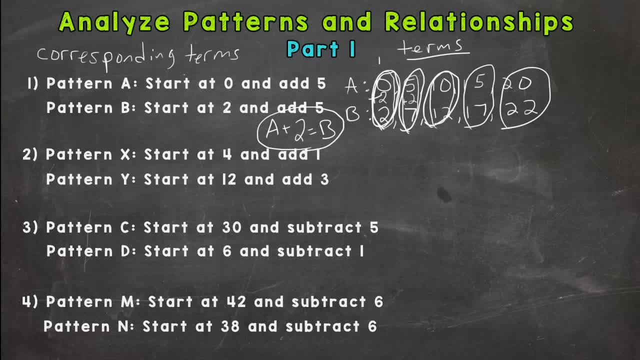 So you can even do the opposite. How do you get pattern B? or go from the bottom to get A? How do you get 2 equals 0? You subtract 2, you do the opposite, so B minus 2 actually equals A, And it will work for all of them And a sentence for that would be the terms. in pattern B minus 2 will go something like this: Pattern B will equal 2.. Pattern B will equal 2.. Better than 2.. Why? Why is there so much 2 here? Now here's an example of this: A and B? Q will be equal from the bottom to get A. A and B Q will equal 2.. How do you? 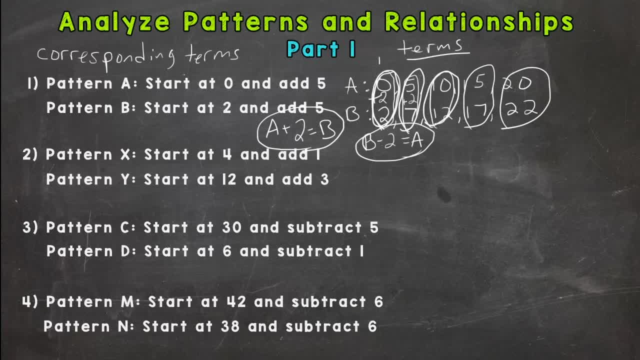 will give you the corresponding terms in pattern A. So let's try number two. here We have X and Y, X, Y. do one pattern at a time, Start at four and add one. So four, five, six, seven, eight. 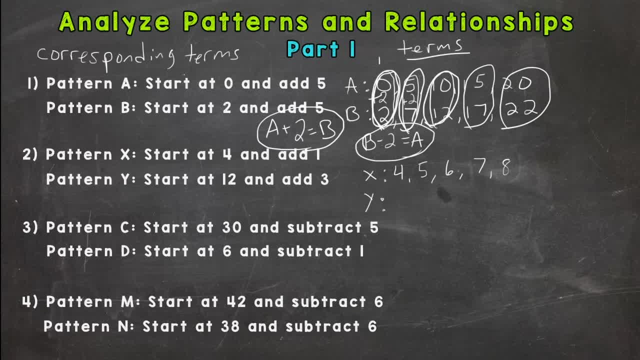 Doesn't get much easier than that as far as patterns. And then we have for Y, start at 12,, add three, 21 and 24.. X and Y, So notice the four and 12,, five and 15,, six and 18,. 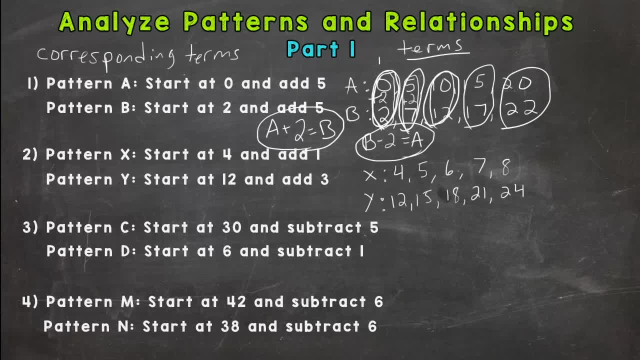 everything's lined up, my terms are lined up, So how do I get four to equal 12?? You might be thinking: well, four plus eight is 12.. But remember you need to check. it has to work for all of them. 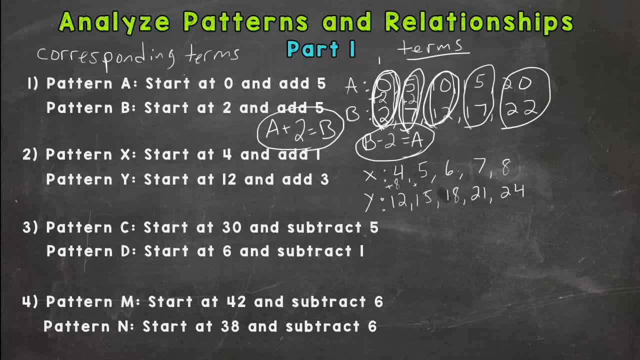 So let's try the next corresponding terms: five and 15.. Is five plus eight 15?? No, Five plus eight is 13.. So plus eight or add eight to X does not work. We need to think of something else. Hint, it's gonna be multiplication. 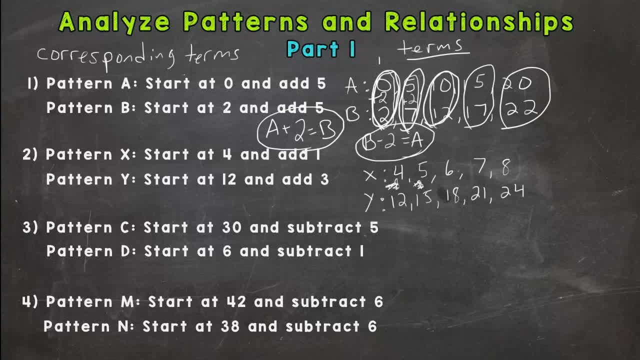 How do I get four to equal 12?? I need to multiply X by three, So three X or three times X gives me Y. Four times three is 12,, five times 15.. Or four times three is 12.. Or five times three is 15,. six times three is 18,. 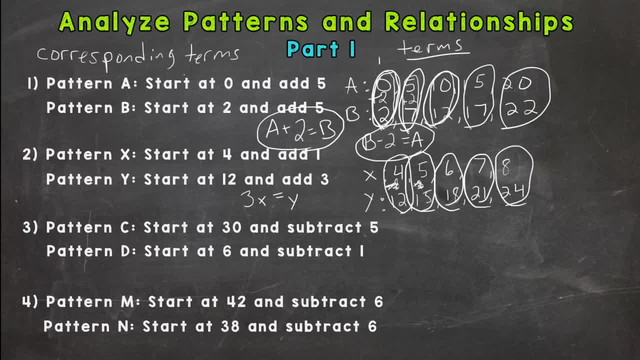 seven times three is 21, and eight times three is 24.. So the terms in pattern X multiplied by three will give you the corresponding terms in pattern Y, Where the opposite would be dividing Y by three to get the corresponding terms in X. 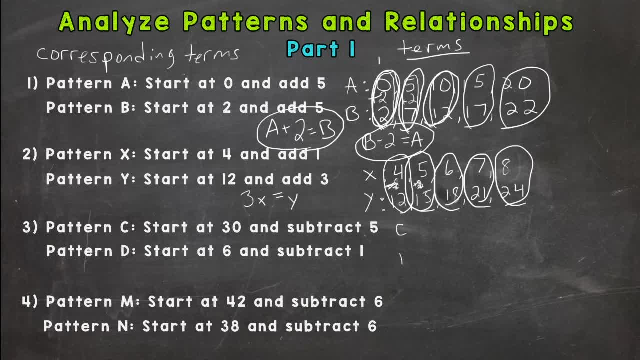 All right, let's do number three. here We have C and D, So we start at 30 and subtract five. Here's our pattern As I write out D- see if you can notice the relationship between corresponding terms. Start at six, subtract one. so a nice little countdown here. 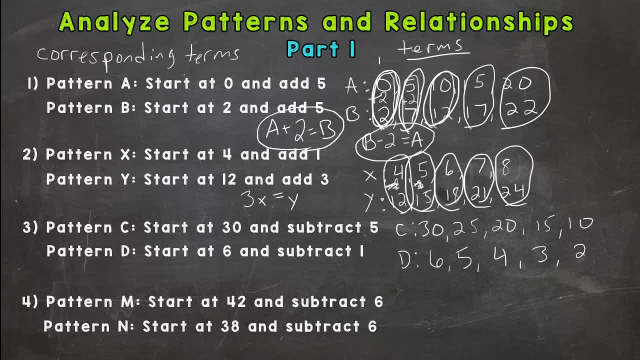 Six, five, four, three, two, All right, so it looks like C. we're starting with 30 and we're going down to six, so we're decreasing in value. So it's either gonna be subtraction or division. Let's try division. 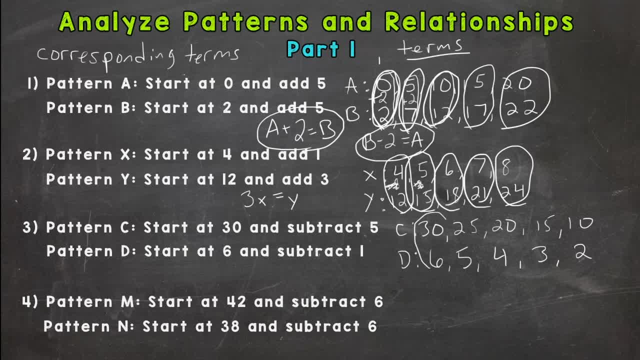 30 divided by five is six. Those are our corresponding terms. Let's try: 25 divided by five is five, 20 divided by five is four, 15 divided by five is three and 10 divided by five is two. So our relationship is pattern C divided five. 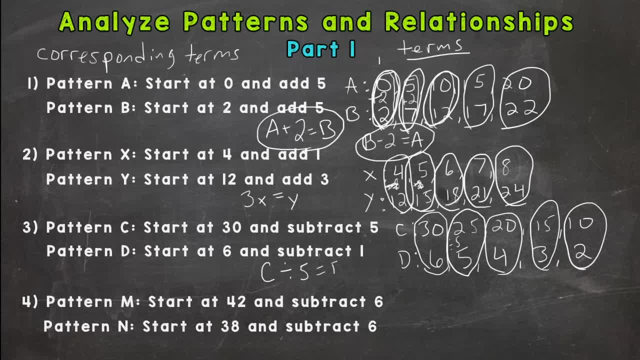 by 5 gives us our corresponding terms in pattern D, or the opposite would be: if we multiply pattern D by 5, we'll get pattern C. remember, a number next to a letter means multiplication, and let's end with number four here. so we start at 42. oh, I didn't label my pattern. this is M and we subtract 6, so 42, 36, 30, 24 and 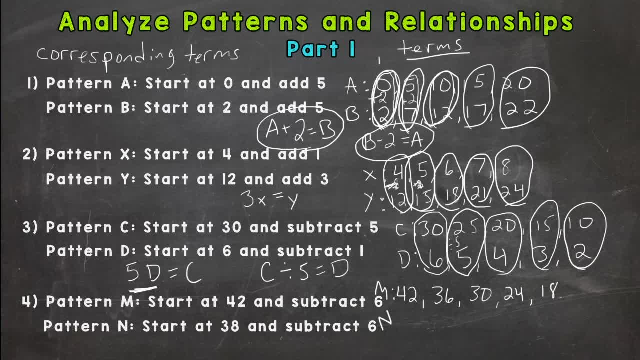 18. and then let's do pattern N and we start at 38 and subtract 6, right, and it looks like we're decreasing from the top going down to the bottom. so it's either going to be subtraction or division, and 42 minus 4 is 38 for our. 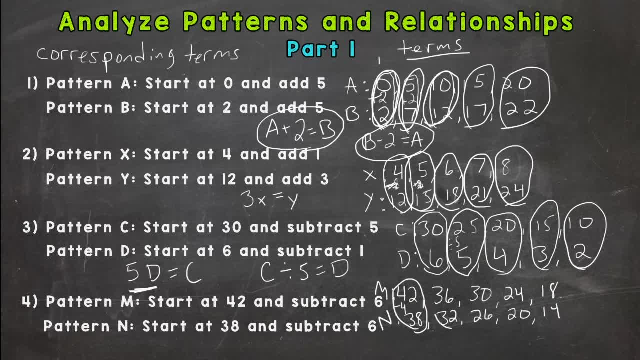 first set of corresponding terms: 36 minus 4 is 32, 30 minus 4 is 26, 24 minus 4 is 20 and 18 minus 4 is 14. so pattern M minus 4 will give us our corresponding terms. and then we subtract 4, and then we subtract. 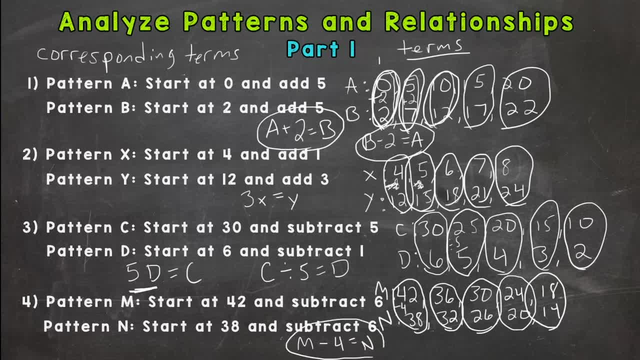 5 to give us our corresponding terms in pattern N. or the opposite, if we go bottom to top n plus 4 will give us our corresponding terms in pattern N. so those, our, those are our four problems where we analyze the patterns and the relationships in those patterns of the corresponding terms. alright, so I'll see.